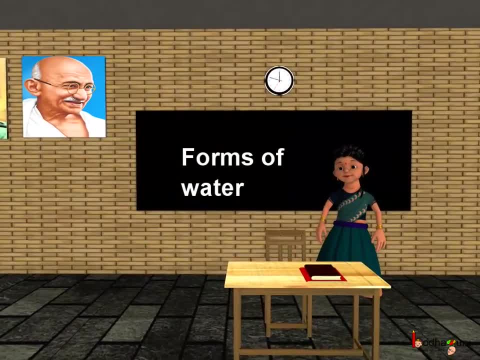 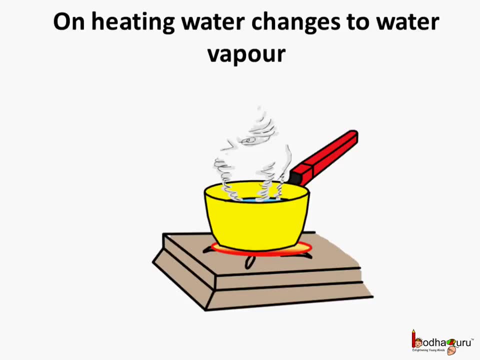 Good morning children. Today we shall learn about different forms of water At home. you must have seen your mother boiling water. And when the water is boiling, what do you see? on the top of the vessel, You see the steam. This steam is also called water vapor. So on heating the water, 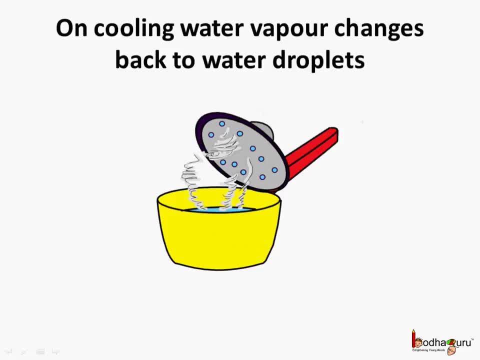 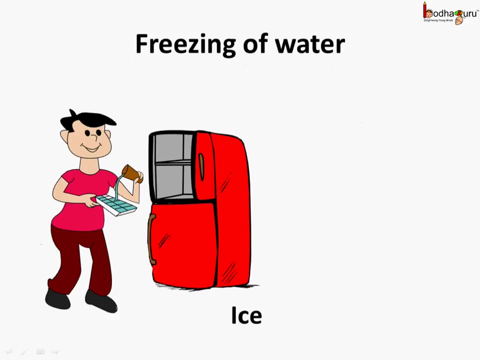 changes into water vapor. Now what happens if we cover the boiling water with a lid? We will see tiny droplets of water on the inner side of the lid. What is it When the water vapor touches the cool lid? it changes back to water. And also, what is ice When we fill the water? 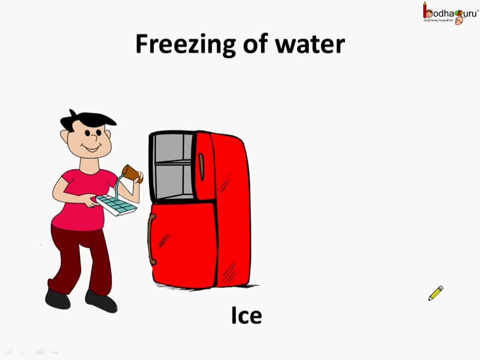 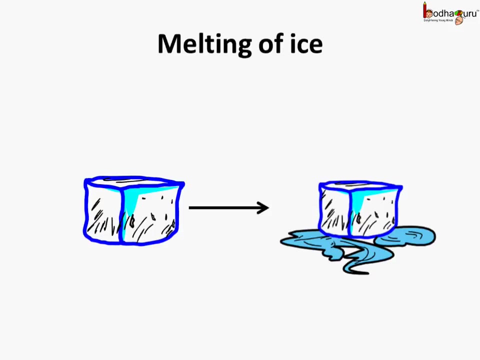 and keep it in the refrigerator. after few hours, you will see ice is formed. So ice is nothing but very, very cold water. And what happens? if we take out the ice from the refrigerator and keep it outside for a long time? It starts melting and changes back to water. 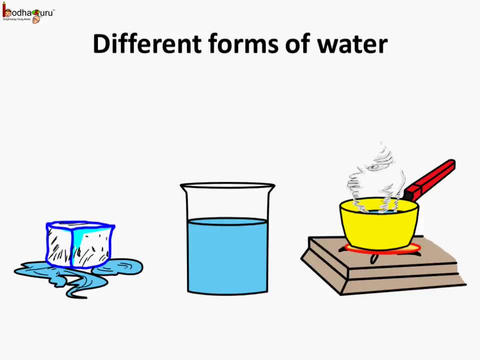 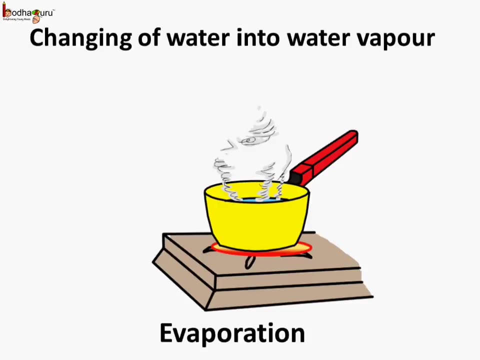 So now you know different forms of water. This is ice, which is very cold, And this is water, And this is water vapor. You know, the process of changing water into water vapor is called evaporation. So remember, evaporation is the process by which, on heating, 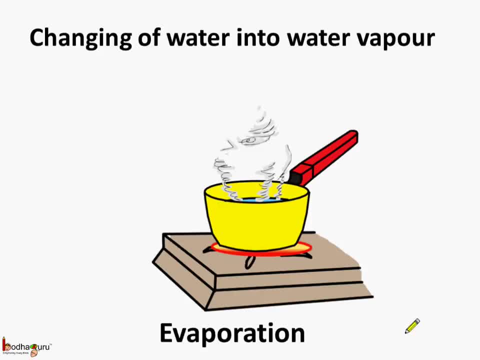 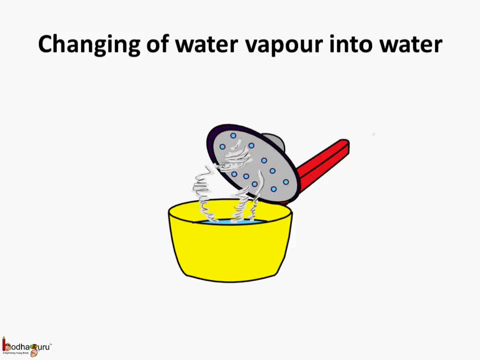 the water changes into water vapor. When water vapor changes back to water due to cooling, it is called condensation. So remember children: condensation is the process by which water vapor changes into water on cooling. So now you know different forms of water. That's all for now. Bye-bye children.